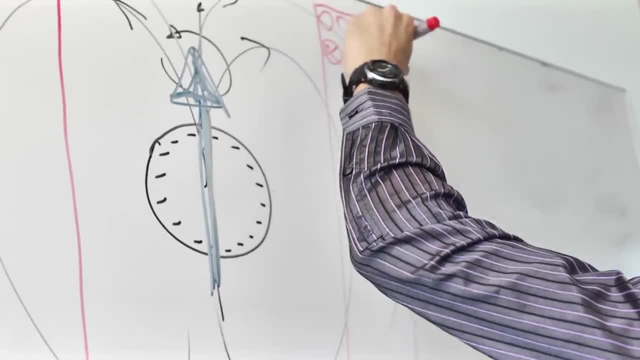 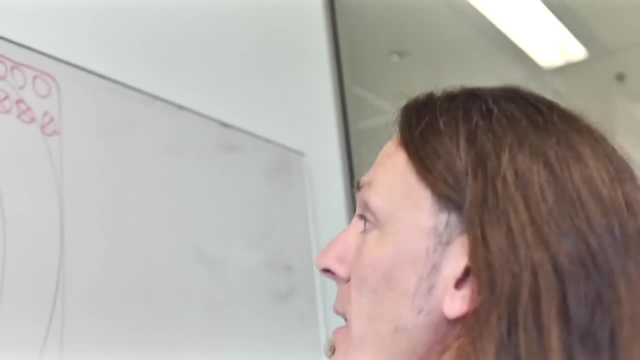 So imagine a solenoid where you have one wires. so on this side you have current going in and on this side you have a current coming out, So you have the current going this way. That produces a big magnetic field in this direction. 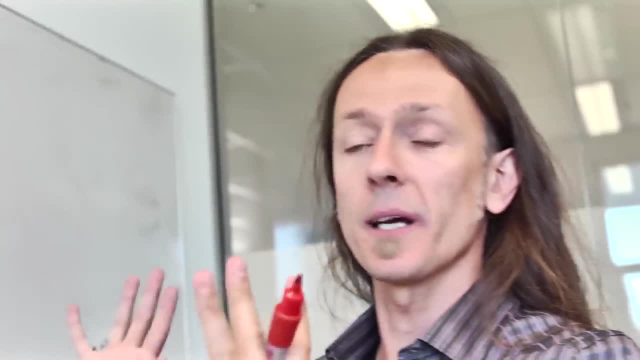 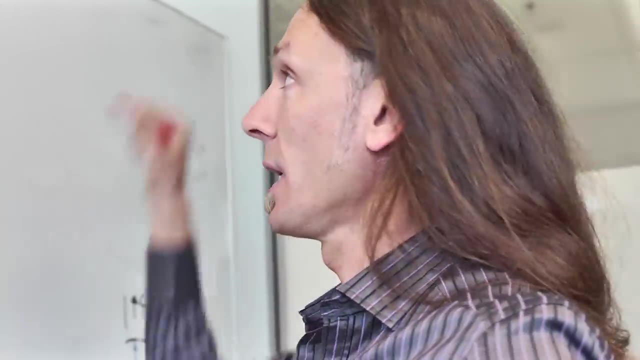 Okay, So that's what we call the b zero, That's the static magnetic field that is produced by us by connecting a large and running a current down this solenoid. So in our laboratory we work with fields of about 1.5 Sidamets per second. 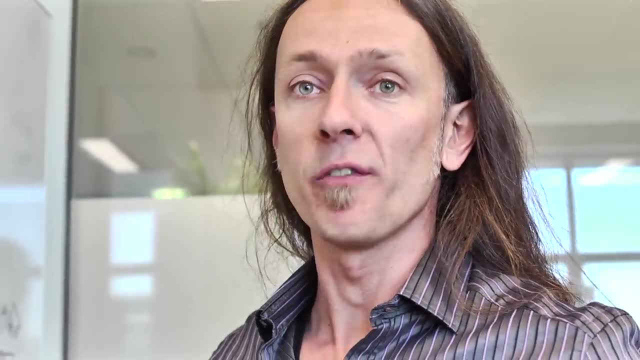 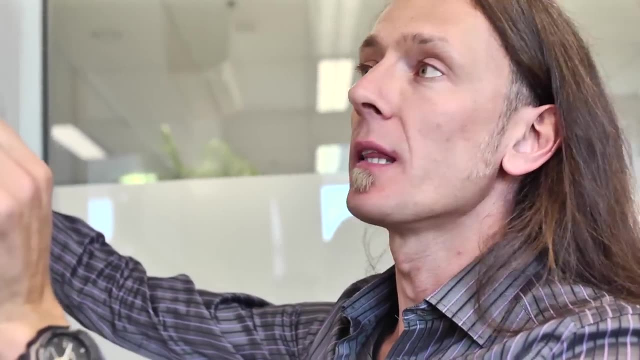 Kundalini by doing that. So this is a good. Actually, we can call it Big verses. Even Milton Tech Do we need to do all that Tesla, which is a strong field? in fact, we have superconducting magnets in this magnetic field, the magnetic dipole that is associated with the spin, with the 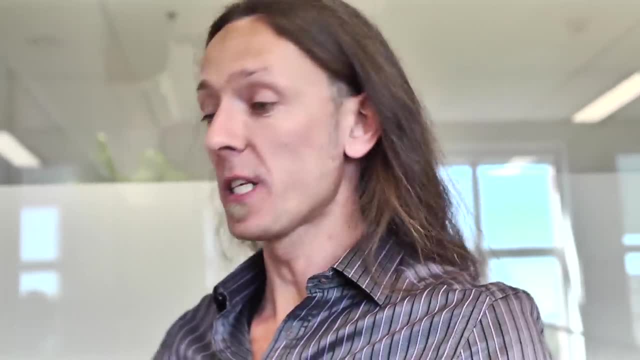 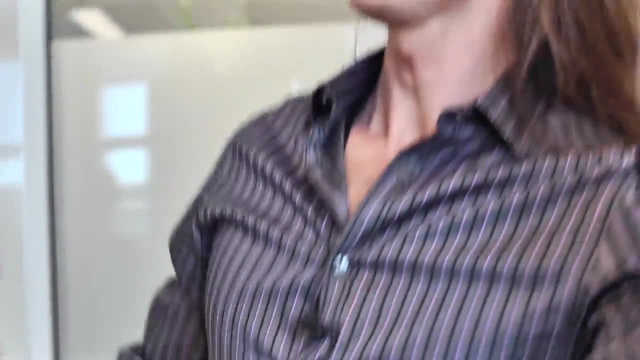 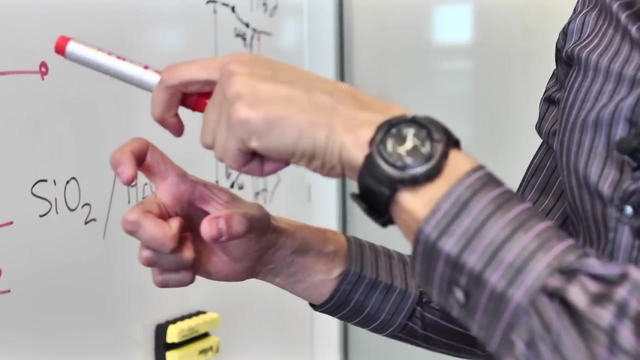 particle will have its lowest energy when it's pointing along the field. okay, think of the needle of a compass, literally. okay, the earth's magnetic field is oriented towards the north, so when you take your compass, you will see the needle pointing towards the north, because that is the direction where the 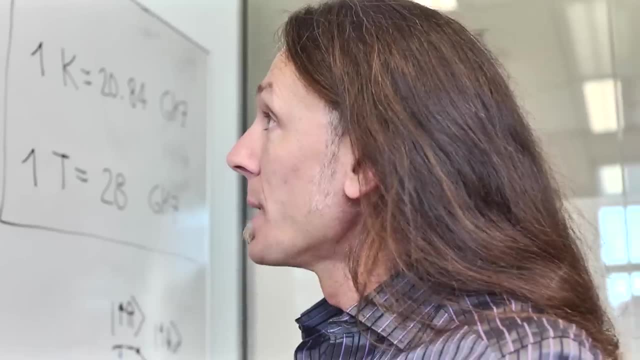 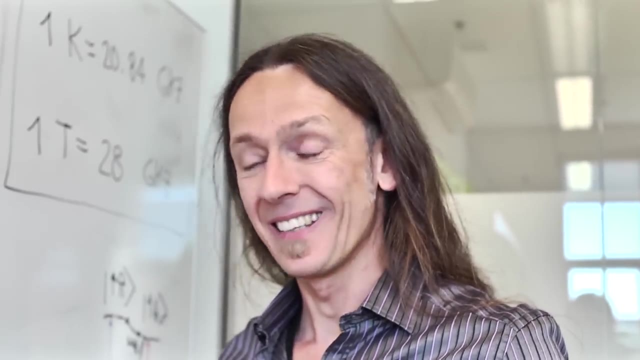 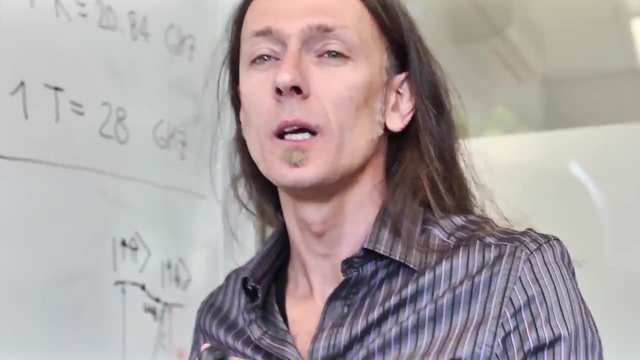 magnetic needle has its lowest energy. okay, but the point is, the spin is not just the needle of a compass, is not just a switch. the spin is a quantum mechanical object that can be in zero and one at the same time, so you can create what's called a quantum superposition of zero and one. so at the 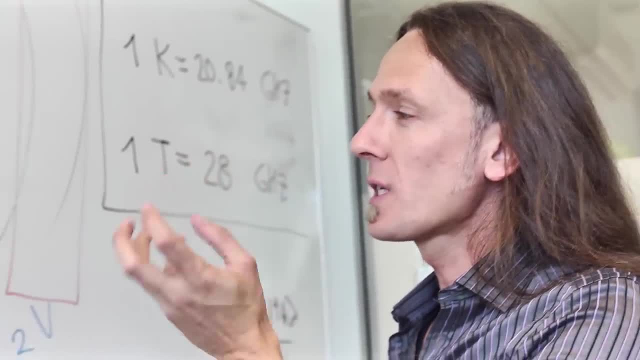 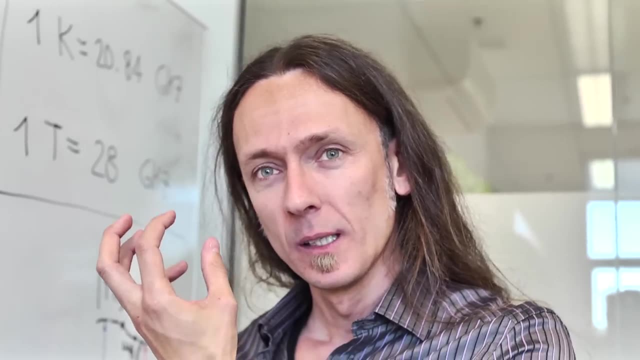 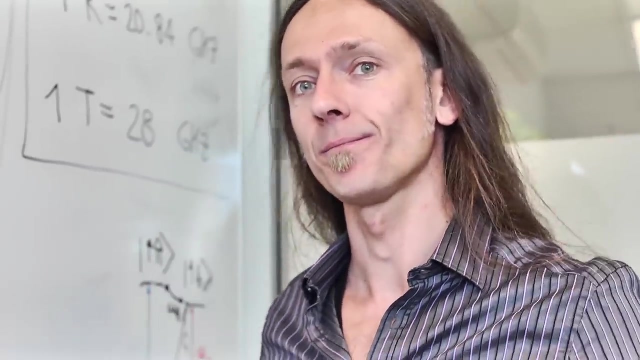 single spin level. it's often hard to see where the quantum mechanical you know you can see where the quantum mechanical you know you can see where the quantum mechanical you know speciality comes in. it's much more striking when you put two of them. then it goes completely out of your classical intuition. let's do it, okay, they could be. 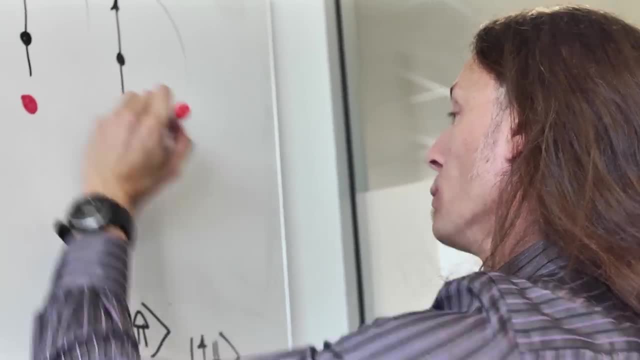 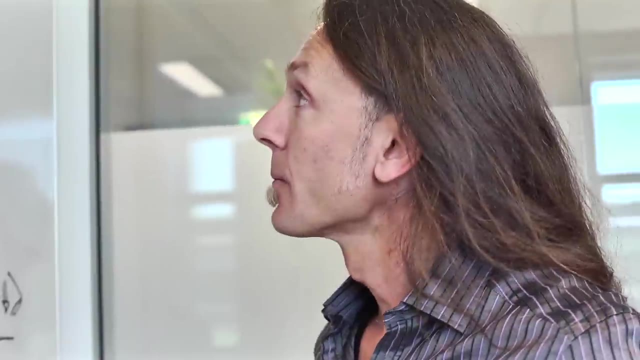 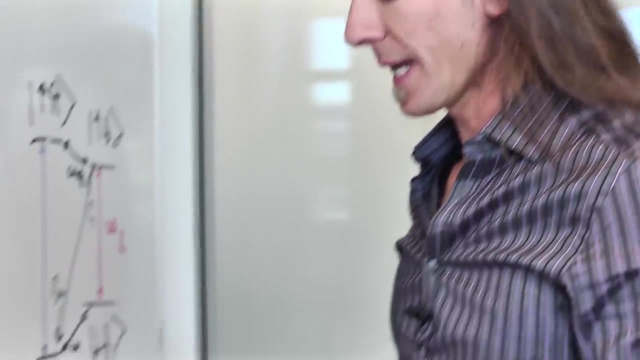 the two electrons that are bound to two different phosphorus atoms. now, when you have two electrons interacting like this, what you'll find is that there are four. I mean, intuitively, you would think there are four possible states. right, that's where you have two electrons interacting like this, what you'll find is that there. 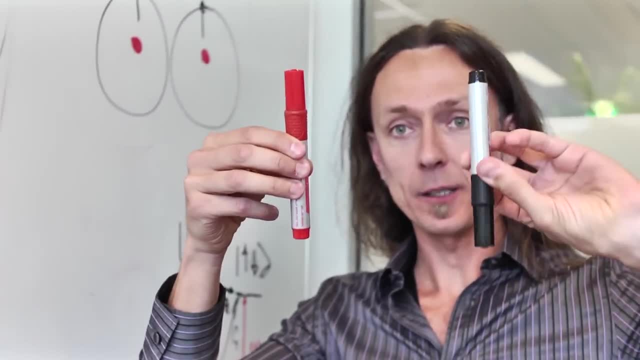 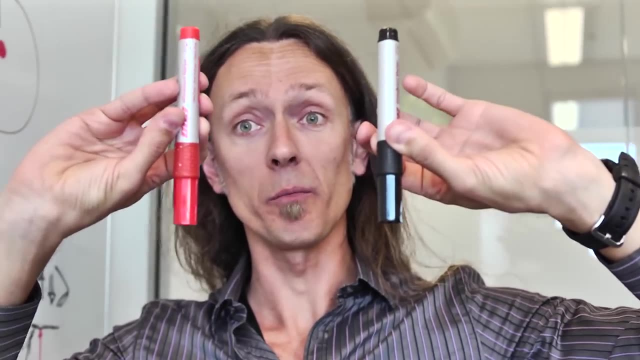 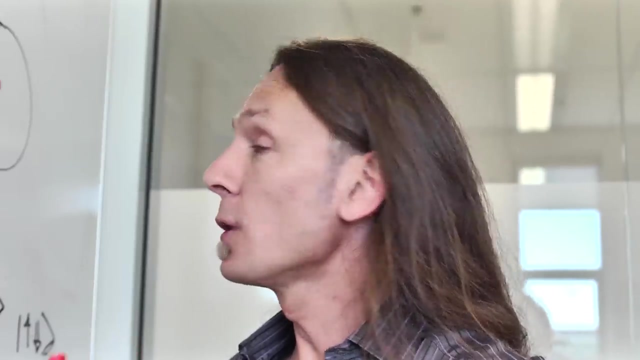 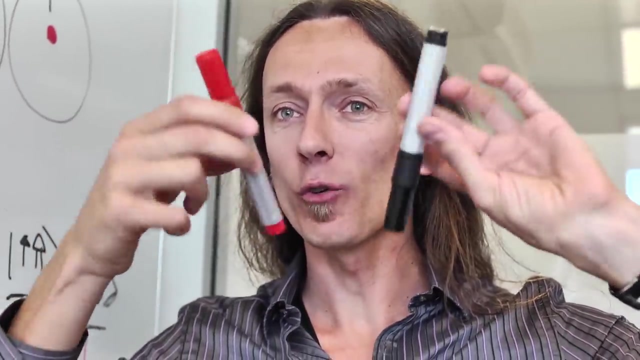 you have electron up, electron up, electron up, electron down, down, up and down, down, right? you think that those are the four possible combination of those two spins. in reality, what you'll find is that you have the up, up and down down. that's fine, but up down and down up are not the natural quantum states of those. 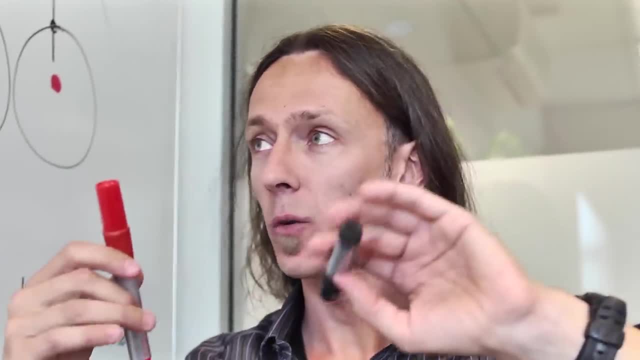 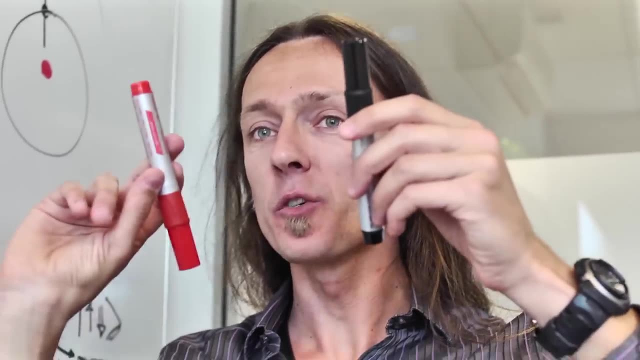 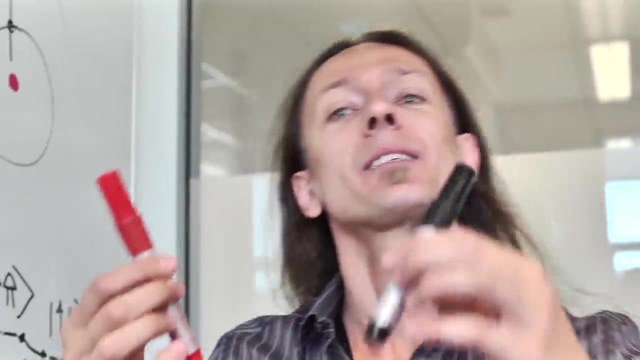 electrons. those electrons will find themselves in what we call the quantum, but up, up and down. up are not the natural quantum states of those electrons. superposition of down, up and條, but that quantum super position has absolutely no classical, intuitive picture to it, in this case this quantum. 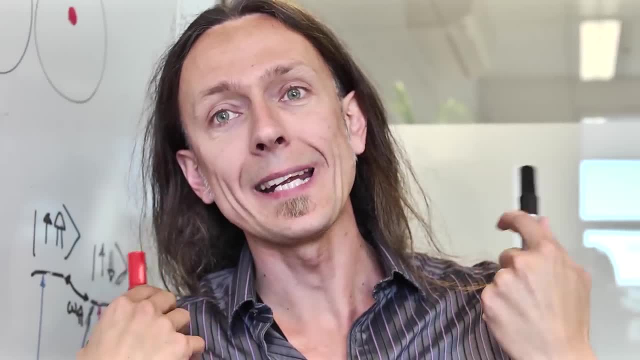 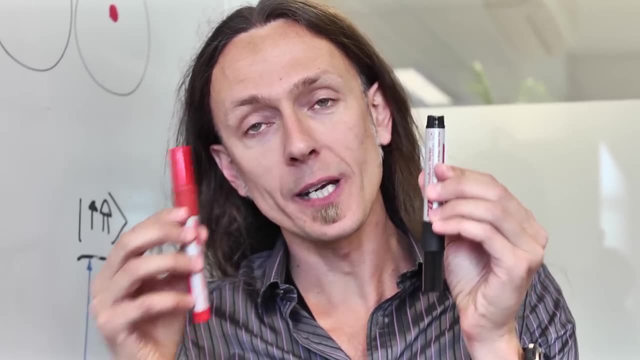 superposition of up, down and damals. up is what we call an entangled state. the superposition of up, down andidel. now not say these electron is down and these electron is up. the two electrons no longer have a direction of their own. so you cannot say this electron is down and this electron is up. the two electrons no. 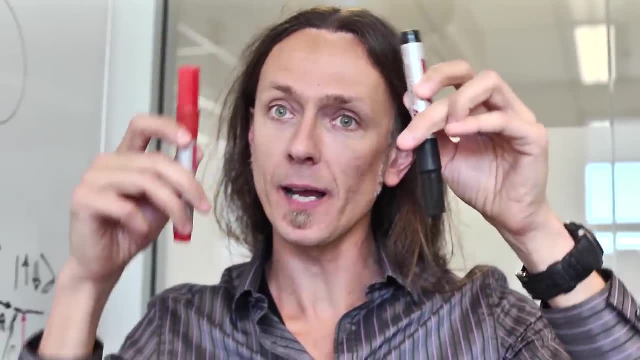 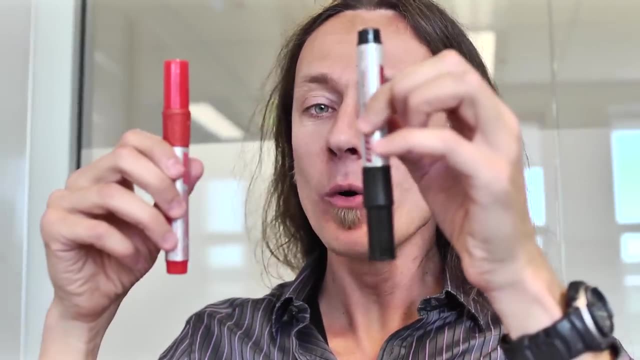 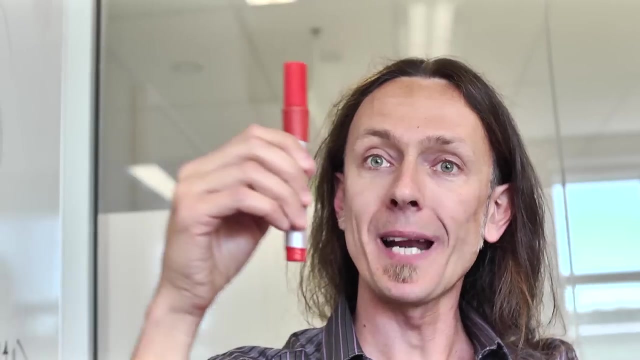 electrons are in a state where they have the opposite direction, but they do not have a direction of their own. so it's only when you measure one of them and you find, okay, this is down, that this one ends up being up. but until you measure them, they are in a state where their only property is being opposite to each. 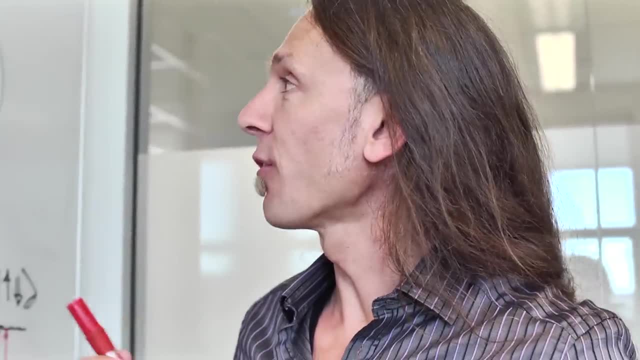 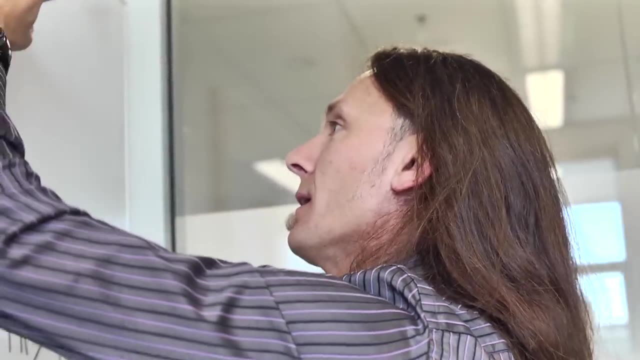 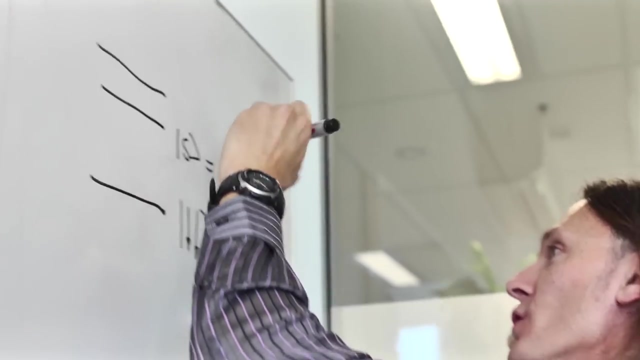 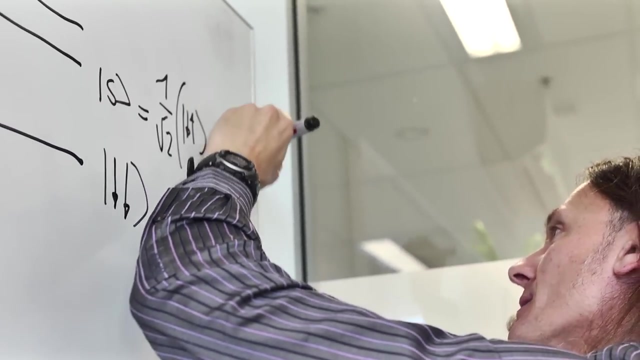 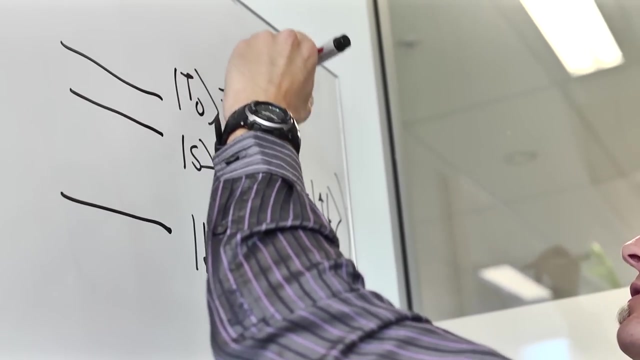 other. why is this so powerful? it's powerful because now you have these four quantum states. right, you have the down down. then you have this thing that we call the singlet state, which is 1 over square root of 2 down up minus up down. then you have this thing that's called the t0 state, which is 1 over square root. 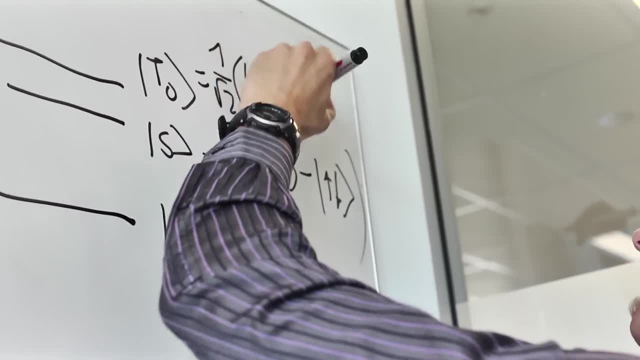 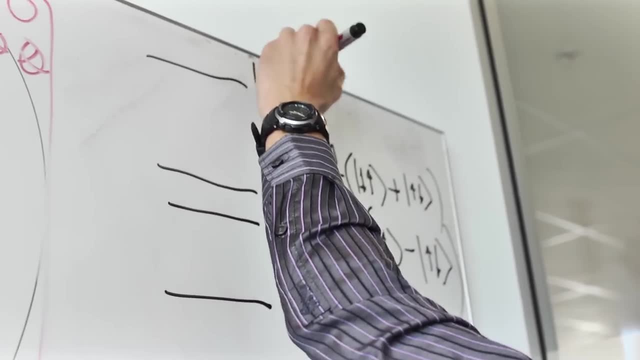 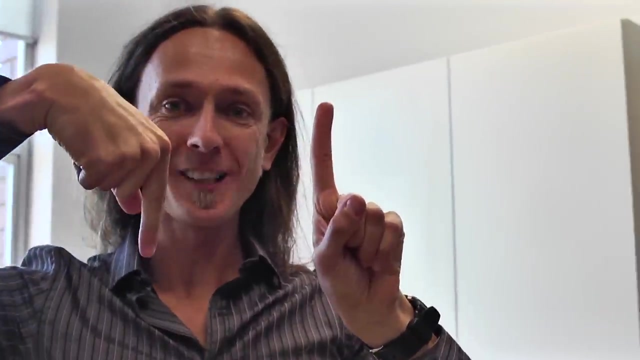 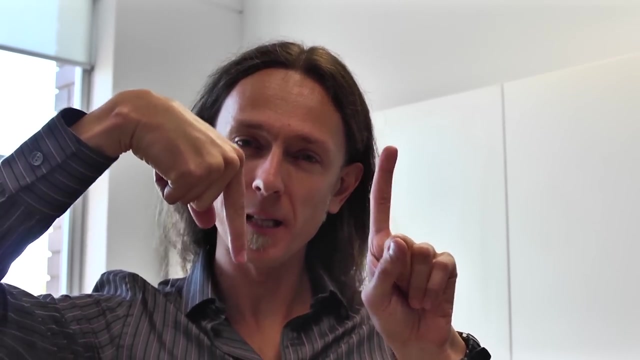 of 2 down up plus up down, and then you have the up up. okay, why is it that the simple up down and down up are not the natural states of the two qubits? that is really where the whole fundamental issue lies: up down and down up are not the natural states. 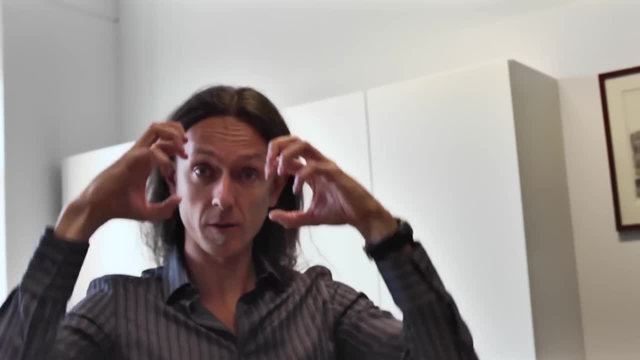 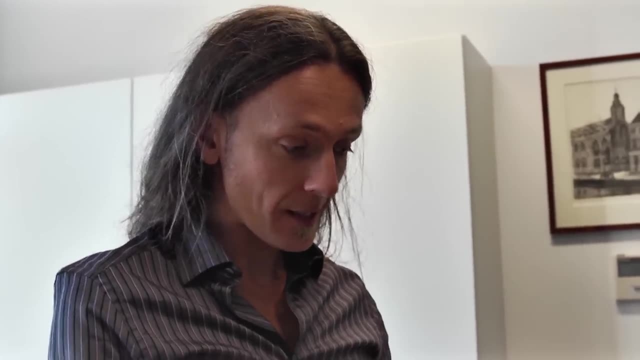 it's because they're coupled. okay, we said we have these two spins. they're coupled to each other. now it's exactly like this double pendulum: you have two pendulums and they're coupled to each other by the string. so let's say I now set one. 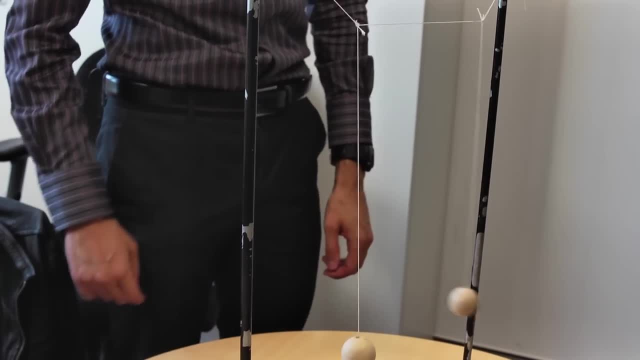 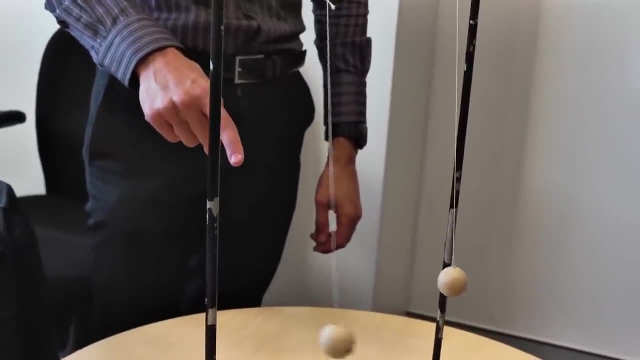 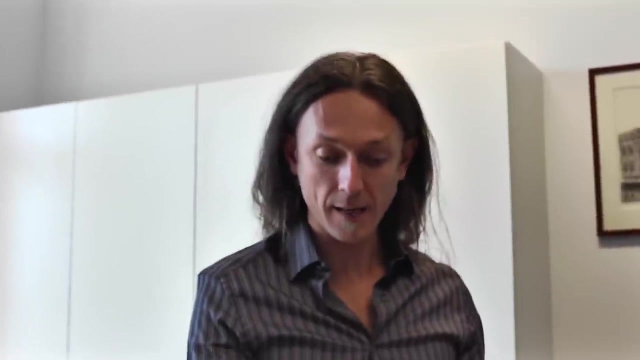 pendulum in motion. look at what happens. you see. now the other one starts to move as well, and at some point- which is about to happen, you see- this one has actually stopped and all the energy is in that one, and then it's going to come back. now, this one. 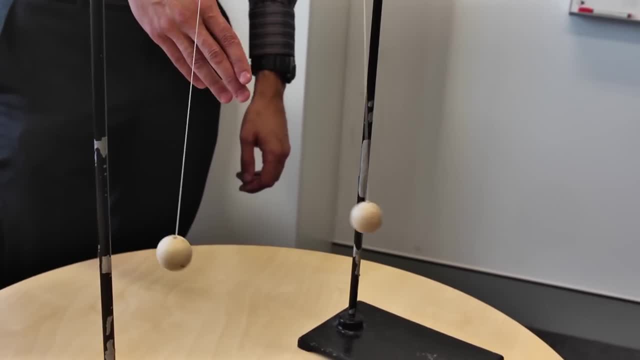 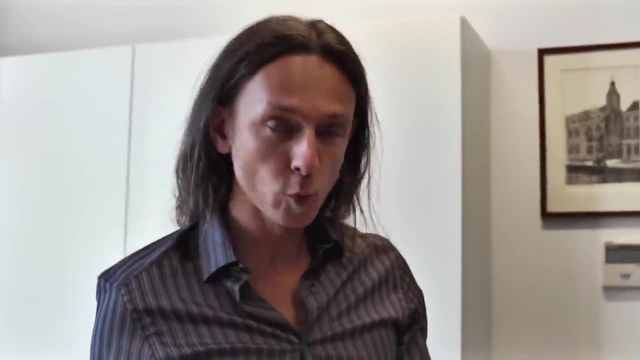 will slow down and the other one will start moving again. so you see, this configuration of the double pendulum is not a stable one, right? so if you just put one pendulum in motion and the other one not in motion, it doesn't stay that way. it kind of. 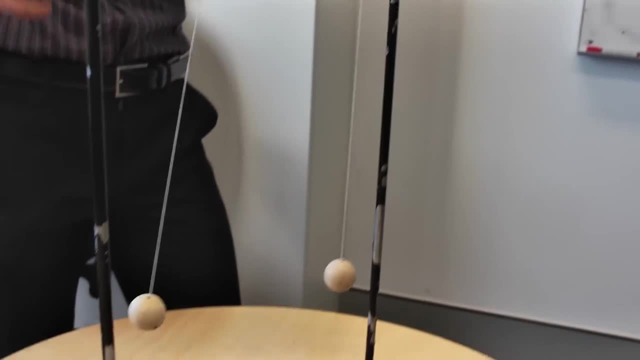 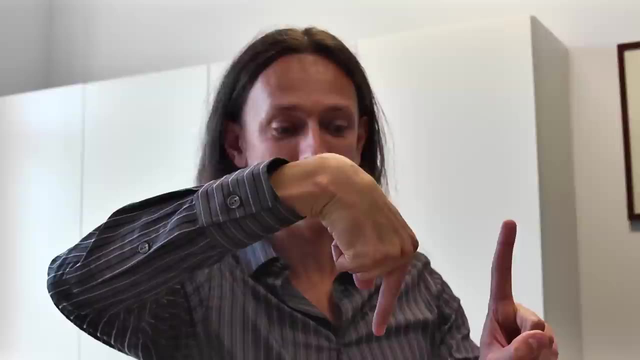 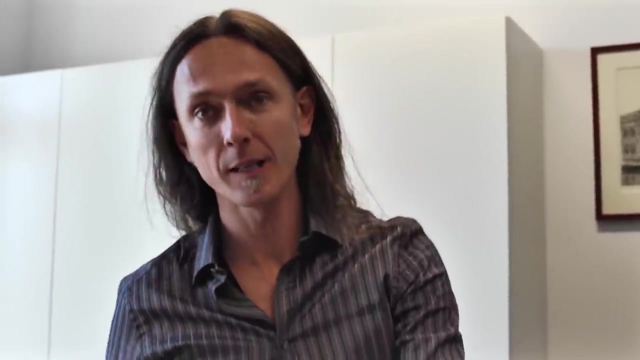 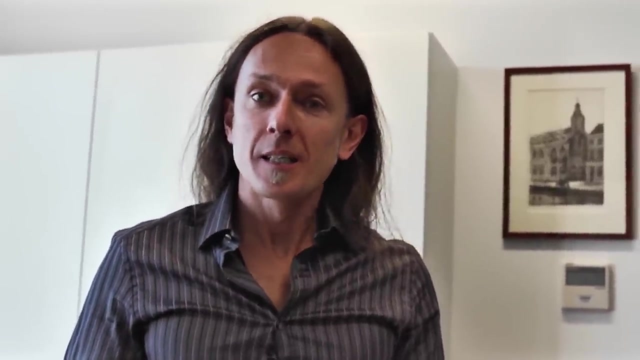 swaps. so you can think as pendulum moving and pendulum not moving, as the spin up and spin down. so if you prepare up down, it doesn't stay there. the up will eventually turn into down and the down into up, like the pendulum that moves, will stop and then the other one will start to move. so then what is the stable? 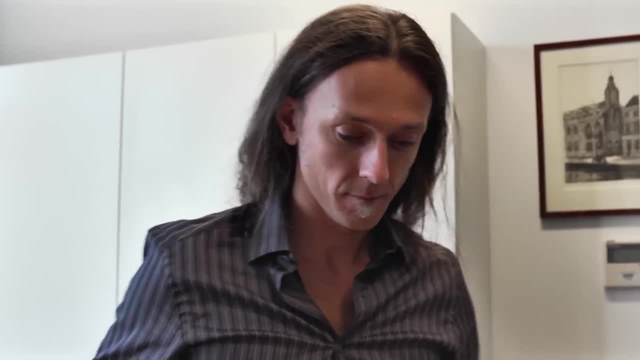 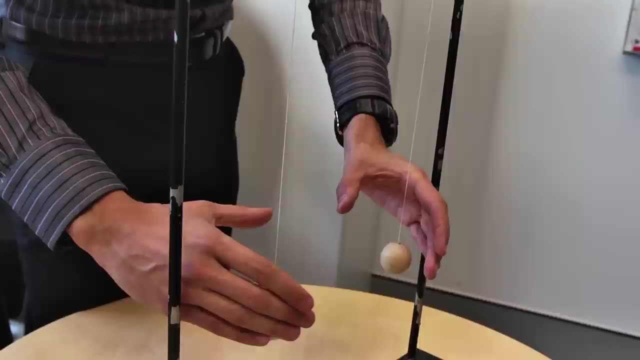 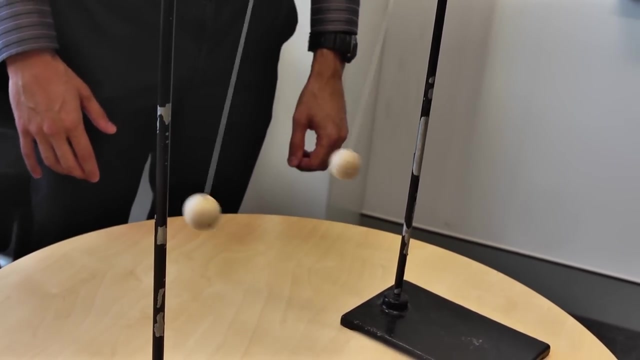 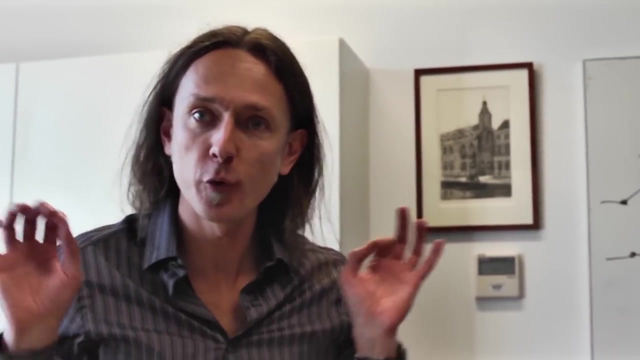 configuration for the coupled double pendulum. well, there is one possibility, which is to put both pendulums in motion at the same time, like this. this will persist unchanged for well, not forever, because the pendulum as dissipation, but if we had a perfect pendulum, this would persist forever. so 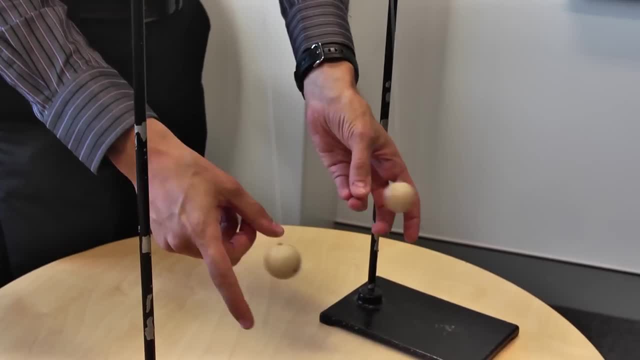 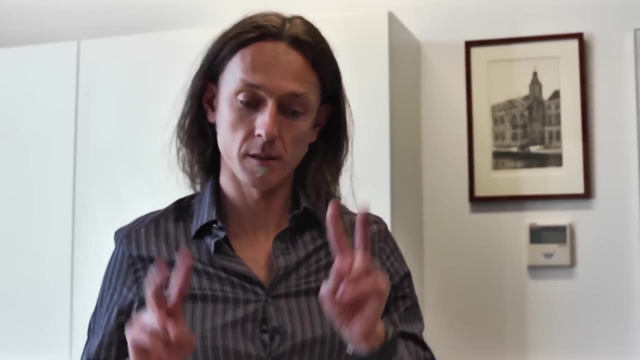 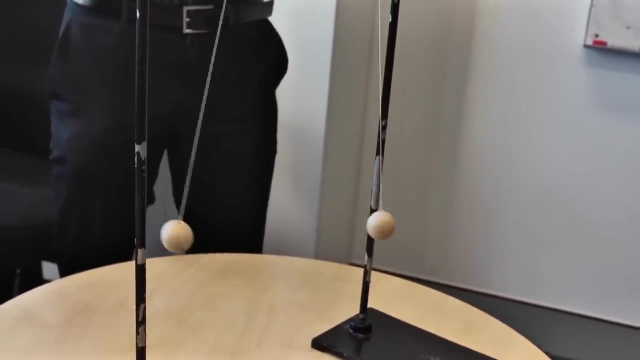 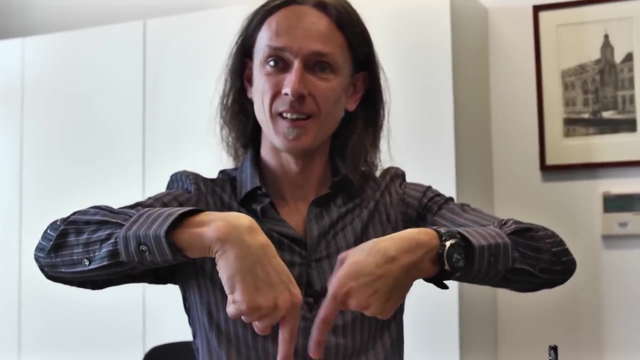 this is one possibility. the second possibility is to do it this way. this configuration will also persist forever, but it's different from the previous one. here the two-pendulum are going in opposite phase, whereas before they were going with the same phase. so that is the meaning of that minus sign that we saw in the two.